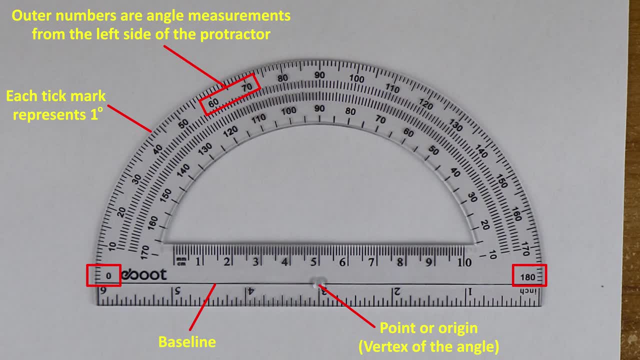 of 10 degrees. here in the protractor are angle measurements, for angles we are measuring from the left side of the protractor. So, for example, this would be a 60-degree angle that I've drawn on the screen And these inner numbers are also angle measurements, but from the right side of 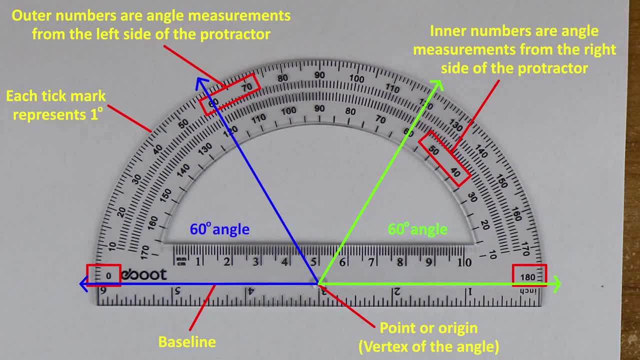 the protractor And here is a 60-degree angle from the right side of the protractor. So these 60-degree angles have the same 60 degree measurement And we use protractors to measure angles and to draw angles. For instance, here is an angle and let's say we need to measure it. 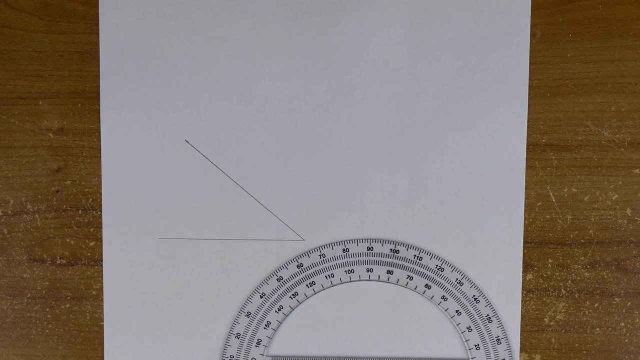 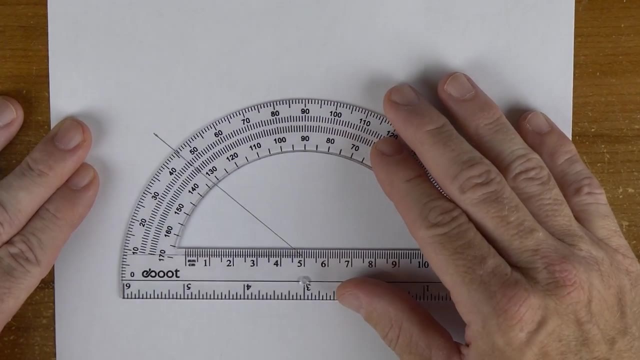 We can measure it from a point of origin, but I will measure only the center point. measure this angle from the right or left side of the protractor. Since the angle opens up to the left, we'll measure it from the left side. We start by lining up the vertex of the angle with the 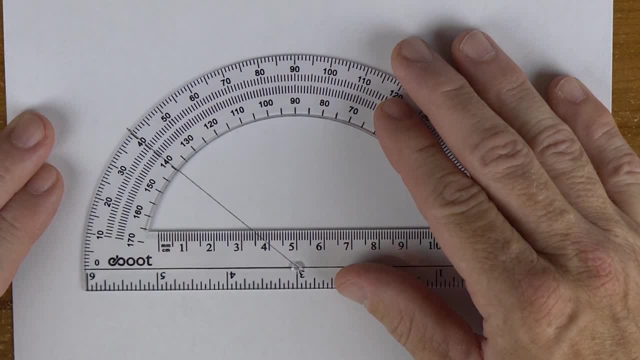 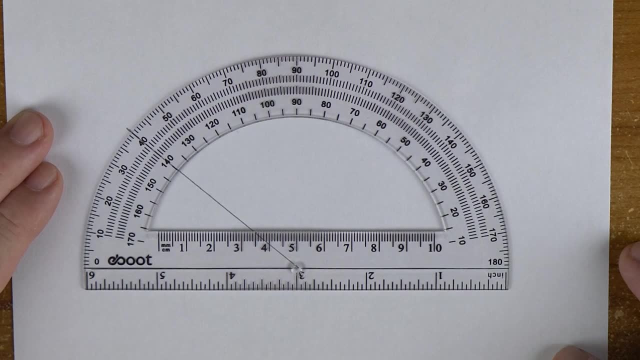 center hole or origin of the protractor and also lining up one of the sides of the angle with the baseline of the protractor, which is a zero degree mark from the left side. From here we look at where the other side of the angle lines up with the outer tick marks on the protractor. You can 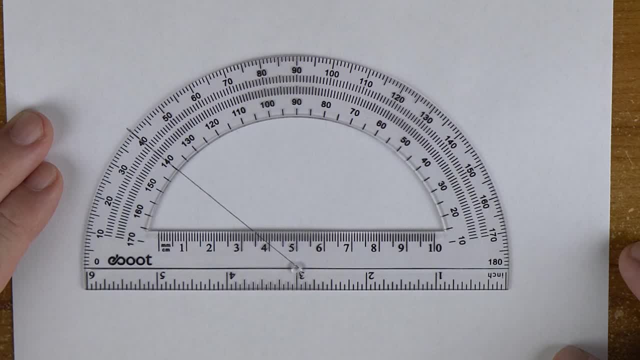 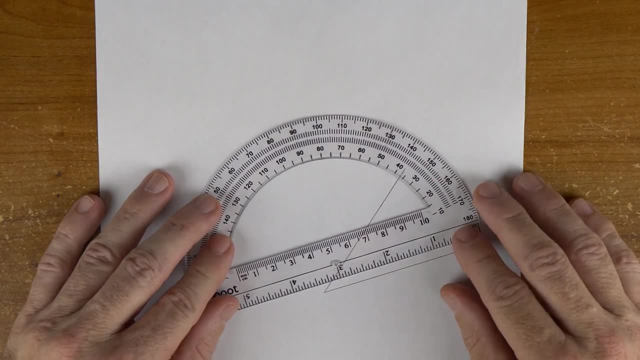 see that this side of the angle lines up with the tick mark at 40 degrees. so this is a 40 degree angle, And here is the same angle, but measuring its degrees from the right side of the protractor. Same method: line up the vertex with the hole, then the side of the angle with the baseline. 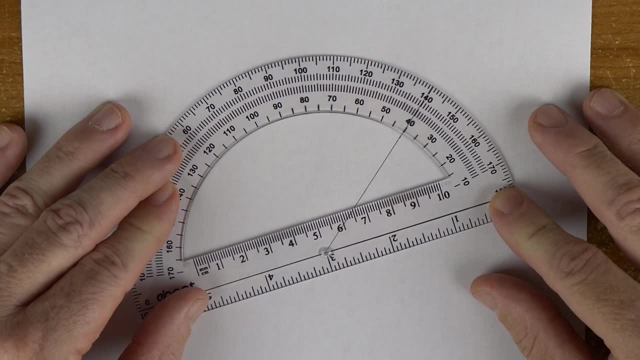 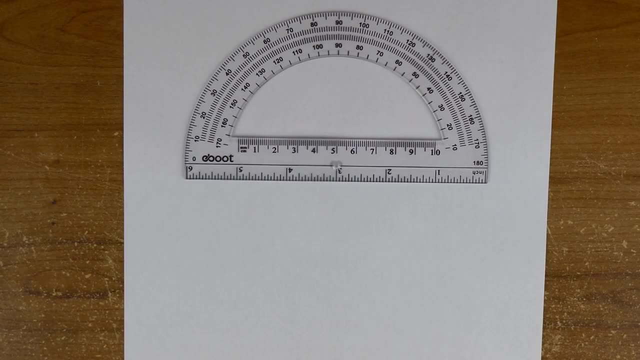 on the right side of the protractor, which is zero degrees from the right side and measuring from the inner tick marks, we get the same measurement of 40 degrees. Now for drawing angles. Let's say that we need to draw a 100 degree angle. We'll start from the left side of 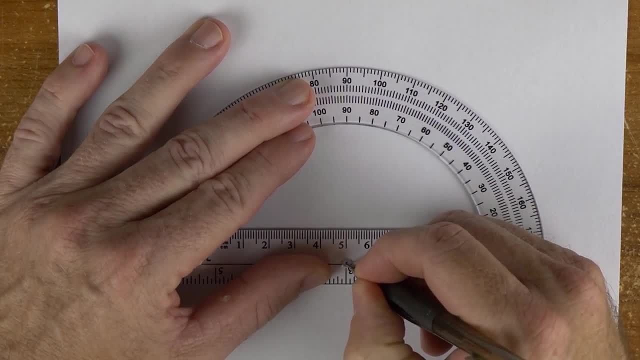 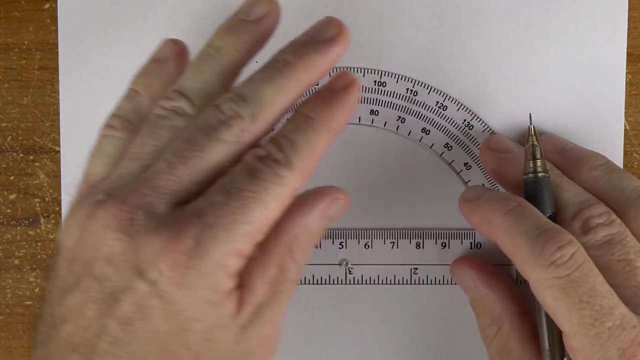 the protractor. We first draw a dot on the paper in the center hole of the protractor. Next we draw a mark on the paper at the zero degree mark on the outside numbers of the protractor to the left. Then we connect the two marks with the straight edge of the protractor. 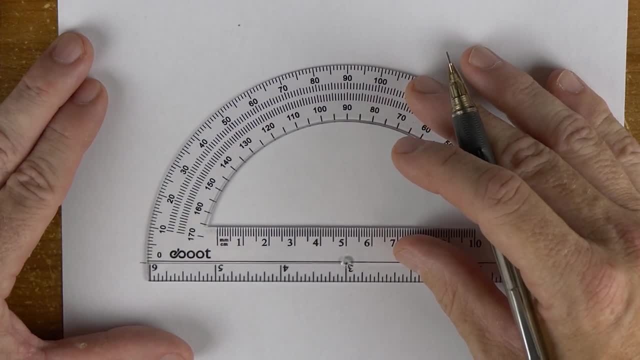 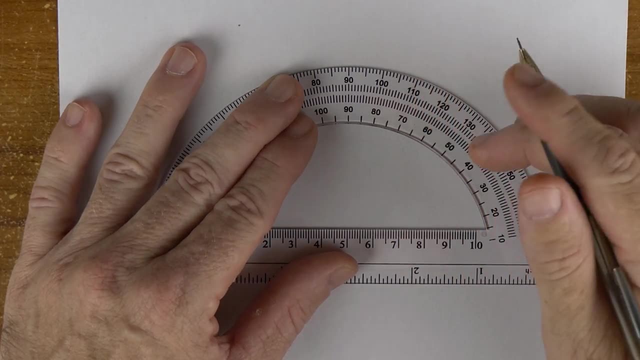 Next we line up the dot with the center point of the protractor and the line we just drew with the left side of the baseline from the protractor. Then we find the 100 degree tick mark on the outside numbers of the protractor and put a mark on the paper at that spot And